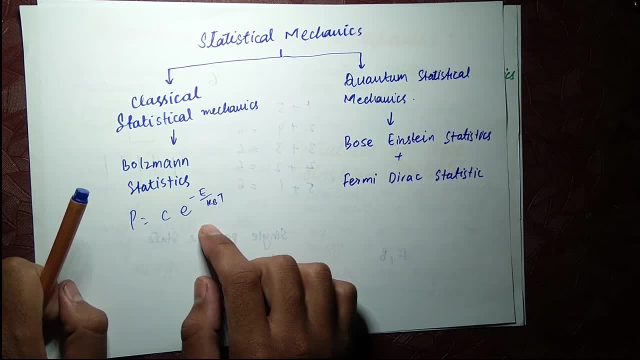 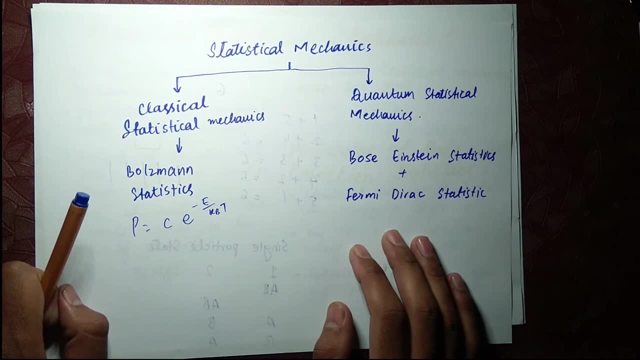 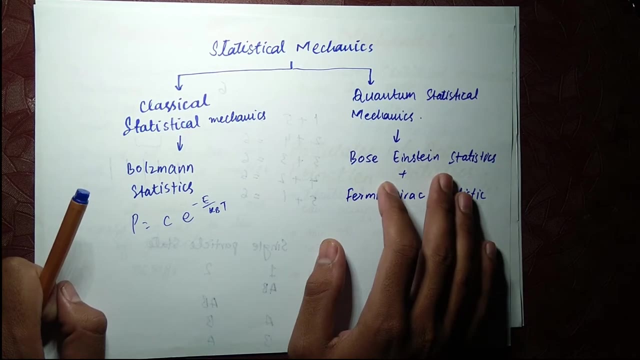 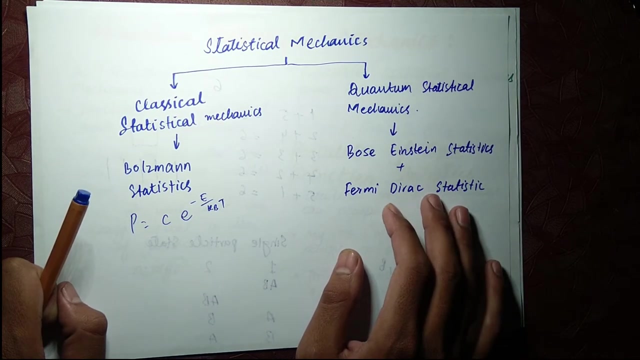 discuss this in detail in our further lectures. so the remaining part was quantum statistical mechanics, which we are going to study today. in this we will study Bose-Einstein statistics and what will be the bosons and Fermi direct statistics, and then we will talk about the fermions. what are they? so let's go. 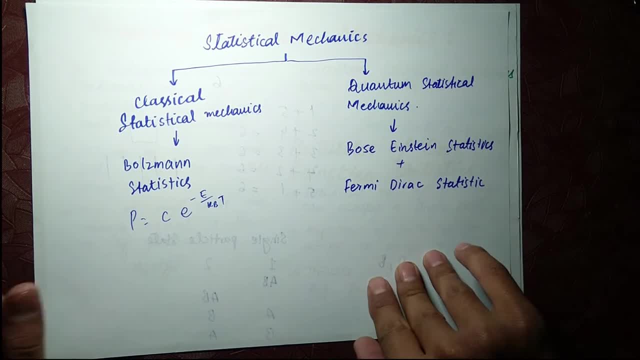 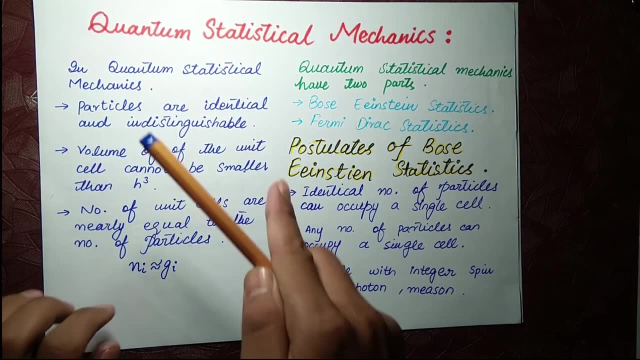 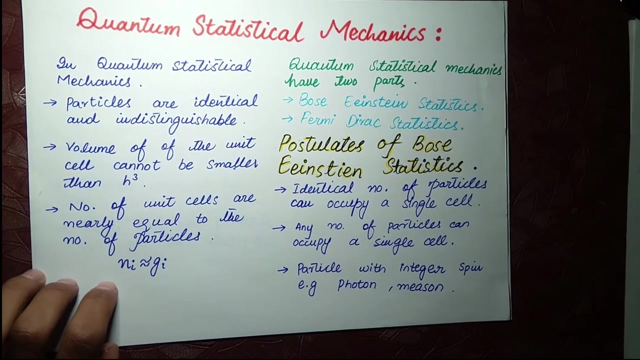 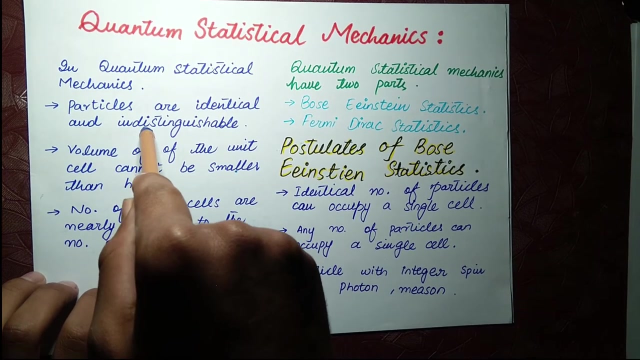 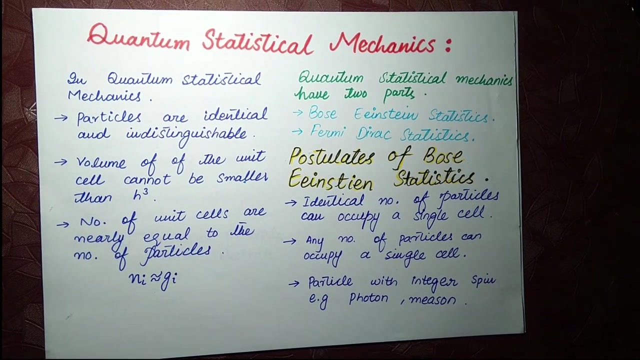 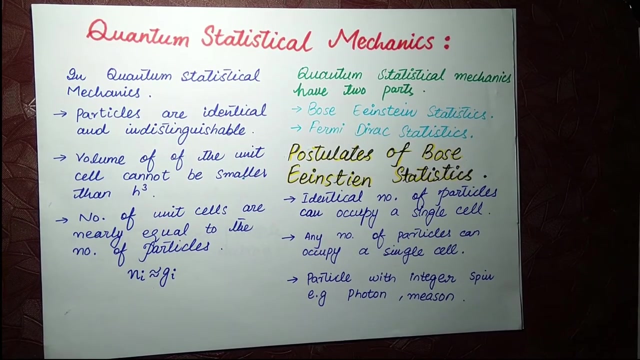 to the quantum statistic statistical mechanics. so in quantum statistical mechanics we say that particles are identical, just like in a classical statistical mechanics. the particles are identical, but in this case they are indistinguishable, we cannot distinguish them. in classical statistical mechanics we can distinguish particles, but in quantum statistical mechanics we cannot. 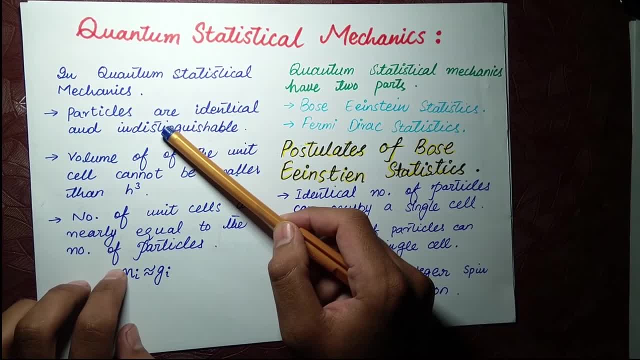 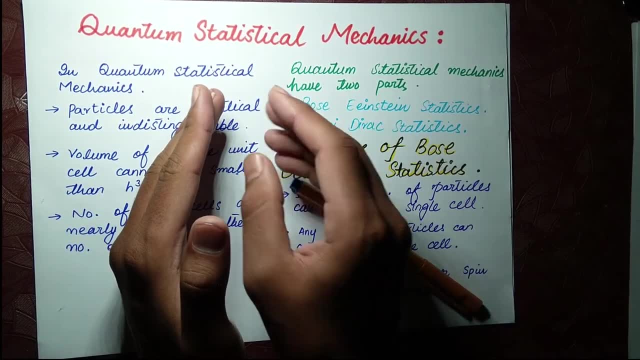 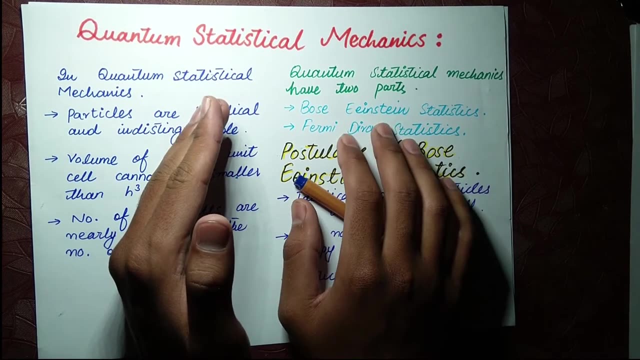 distinguish a particle. for example, in a system we have two particles, so after some time t we cannot say that this particle was a and this particle was B. we cannot distinguish them. they are indistinguishable, they are similar, they are identical. we cannot say that this one 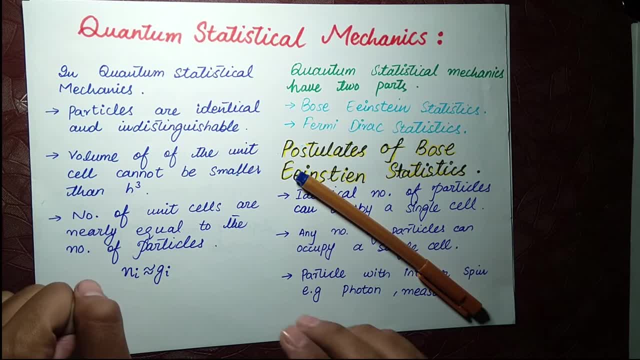 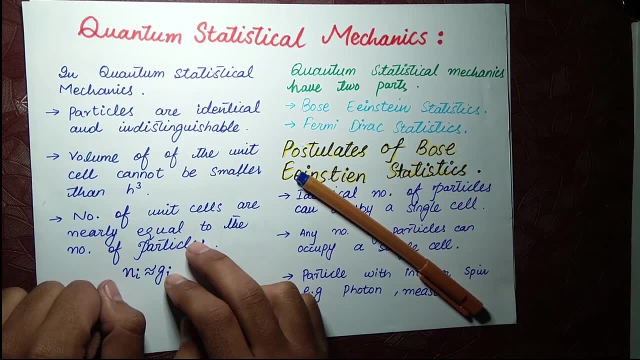 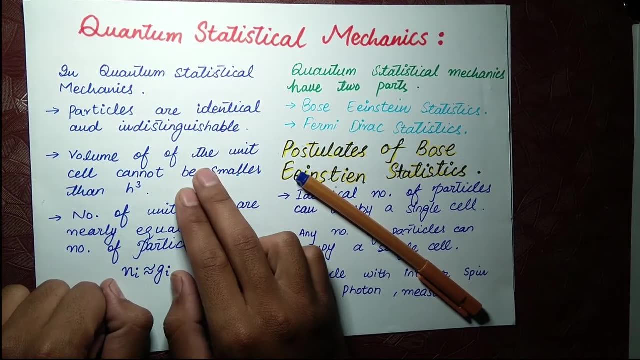 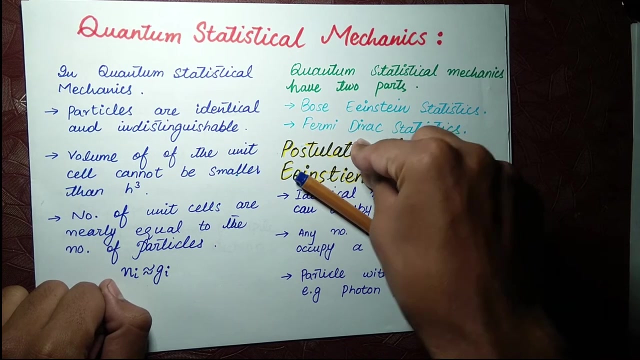 was this and this one was this. so, volume of the unit cell. the next postulate here is that the volume of the unit cell cannot be smaller than H cube. what does this mean if means that when the volume of any unit cell or when the volume of a state becomes smaller than the H cube- H is the Planck's constant- 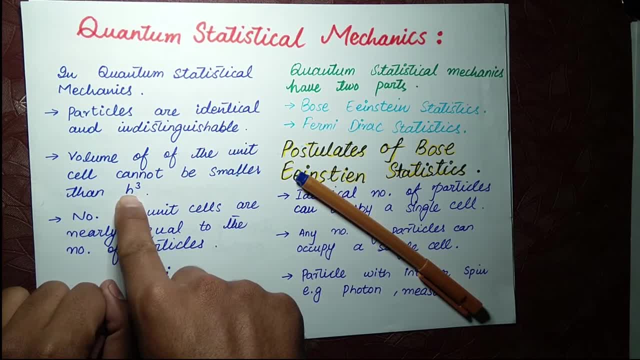 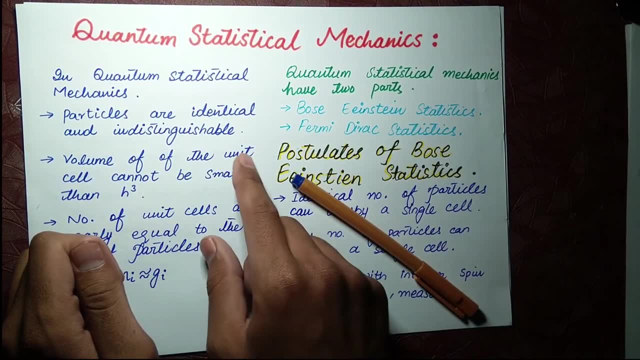 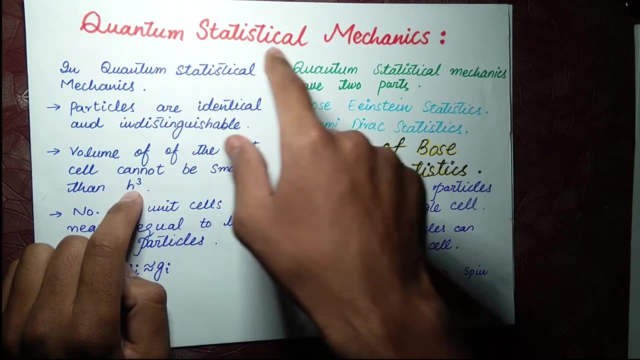 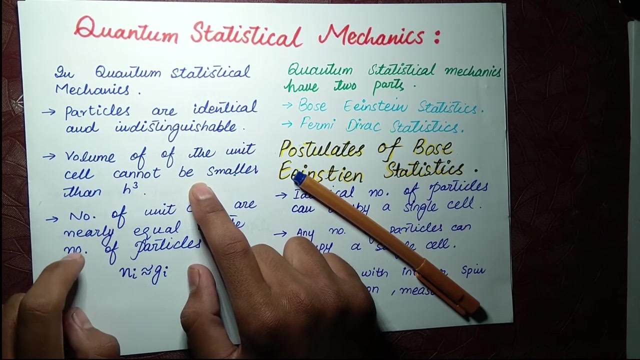 here. and we know that Planck's constant has a constant value. so when the of the unit cell goes to, goes to the value of less than HQ, then our quantum statistical mechanics or our quantum mechanics fails to describe it. okay, so let's go to the next postulate I have. I hope you understand this. so the number 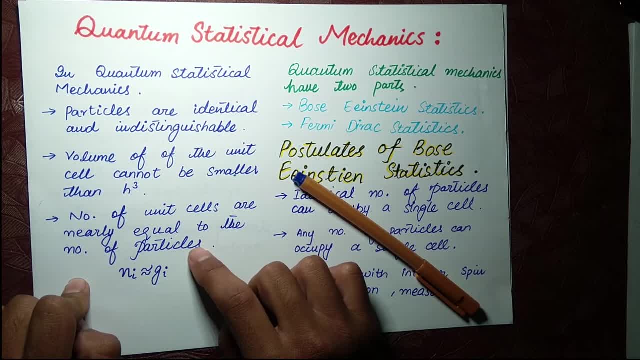 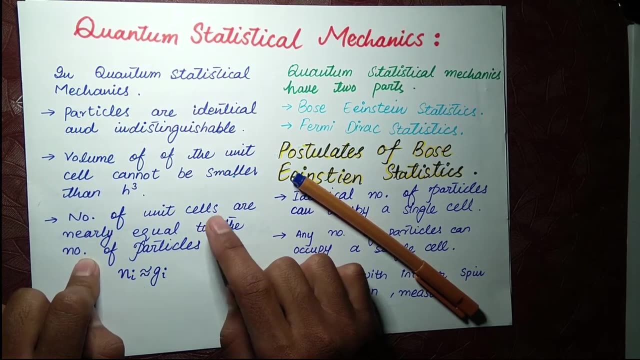 of unit cells are nearly equal to the number of particles. the next postulate is the number of unit cell. in classical mechanics we've said that the number of particles are much, much greater than the number of unit cells, that the number of unit cells are less than number of particles. but in this case, in the 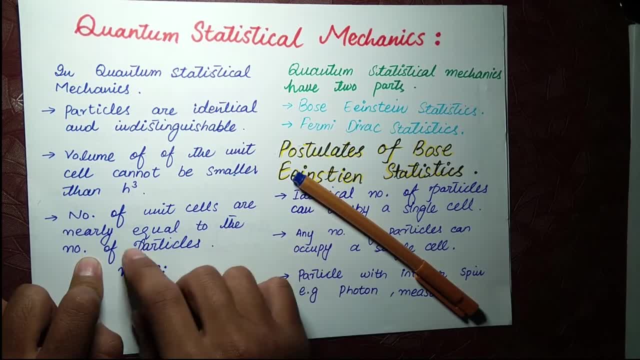 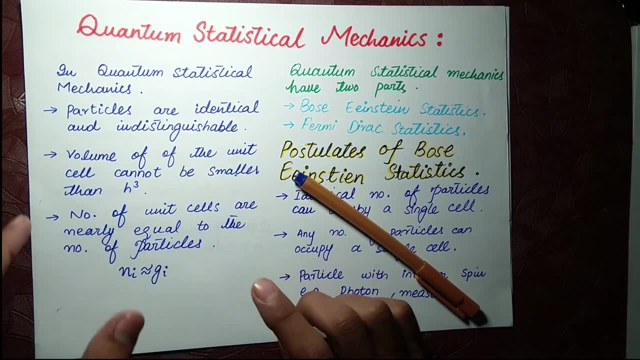 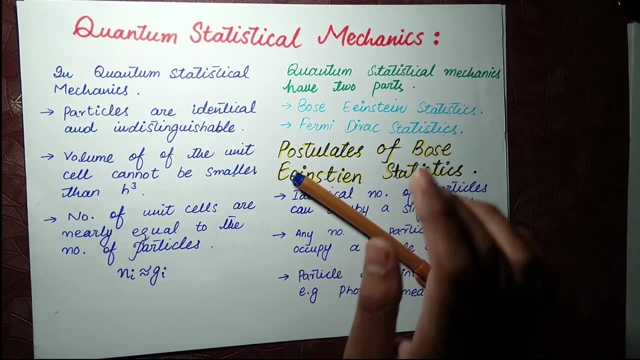 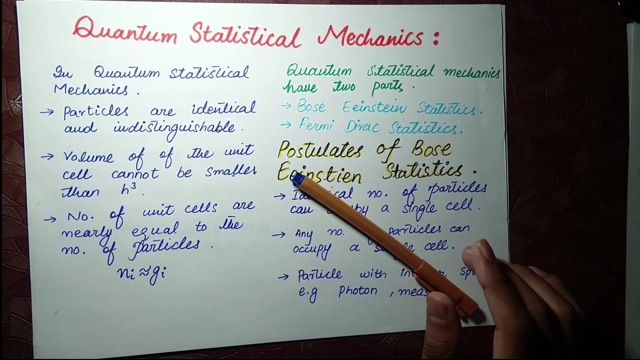 quantum statistics we say that the number of unit cells and the number of particles are same, are nearly equal. so these were the part, these were the postulate in quantum statistical mechanics and now we are going to work the types of all the parts of quantum statistical mechanics. so in quantum statistical mechanics we have 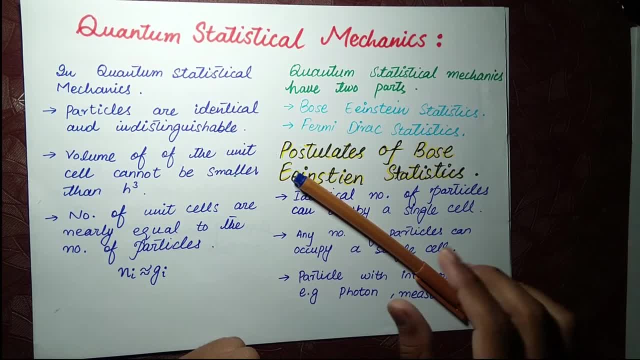 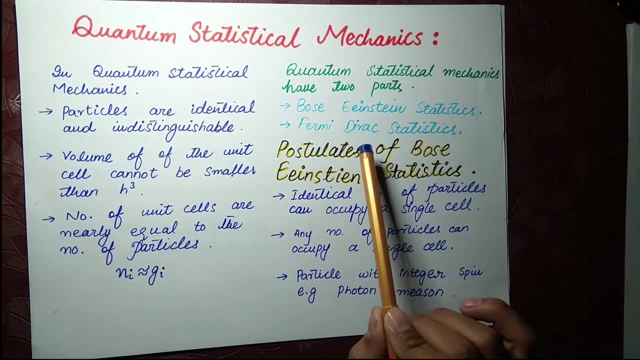 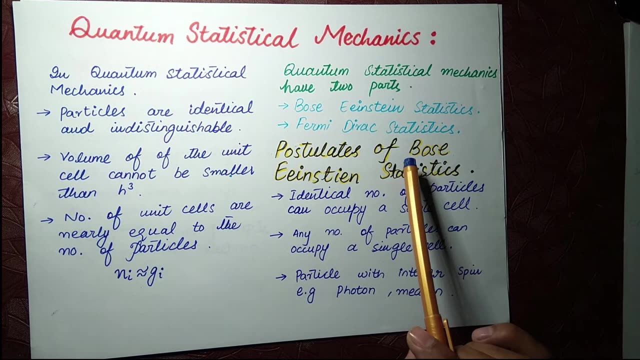 two parts. we have two main parts, and first one is a Bose-Einstein statistic and the second one is the Fermi direct statistics. what is both Einstein statistic? let's see. so the postulate of the Einstein statistic says that identical number of particles can occupy a single. 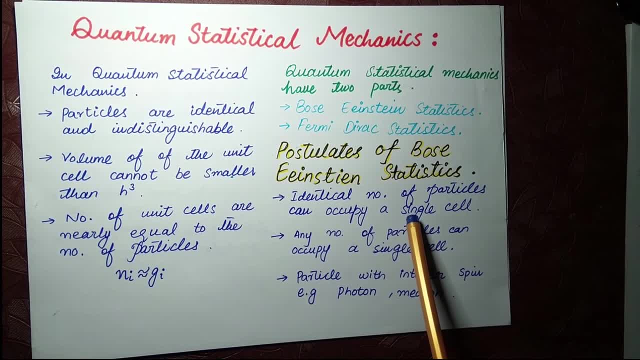 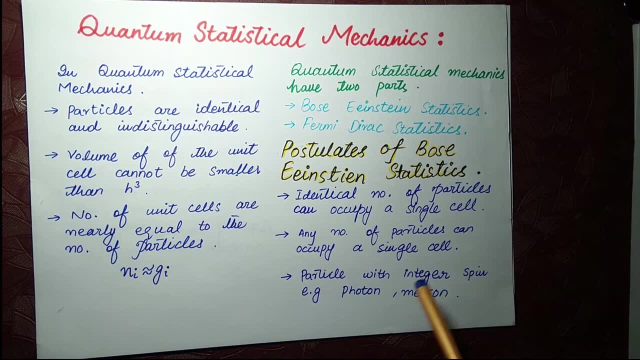 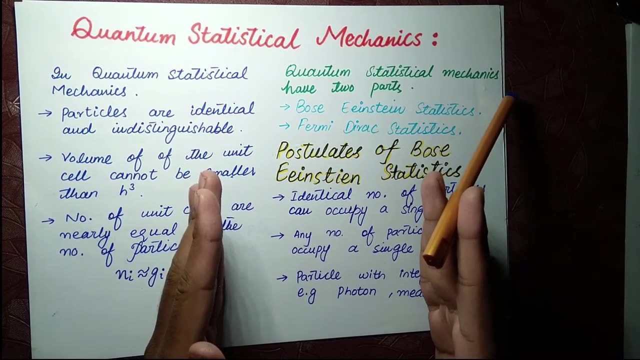 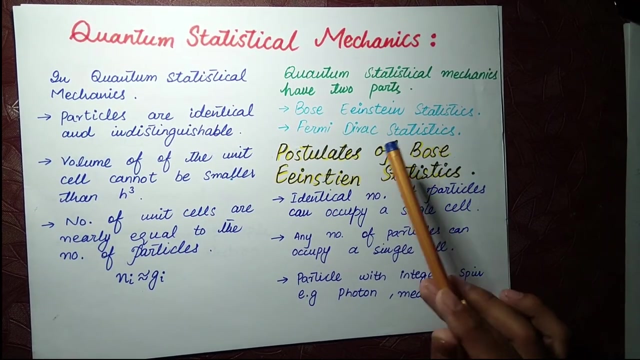 cell identical number of particles can have, because when we look on a bosons, just like photon enemies on, they have similar spin, they have integral spin. okay, and when we will see the Fermi direct, you will see. you will see that if you are interested in learning about quantum évidemment. 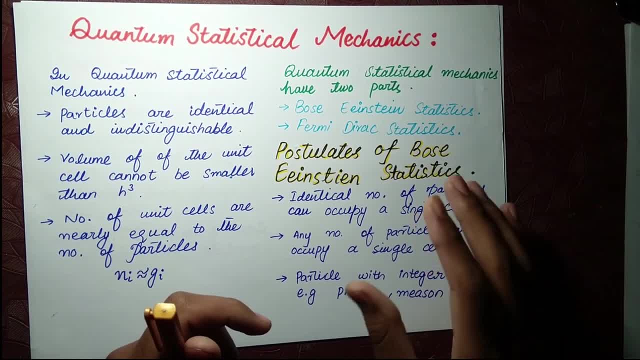 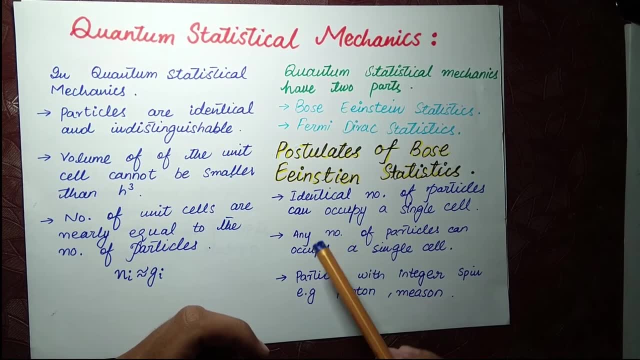 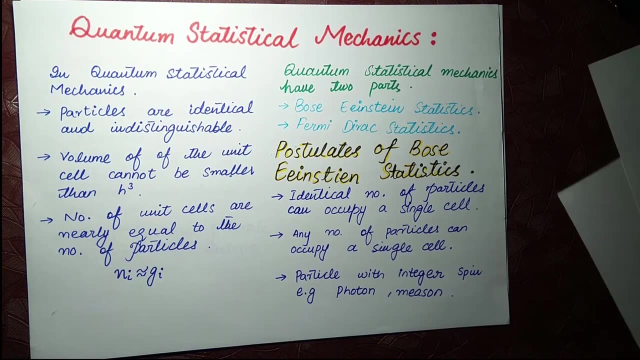 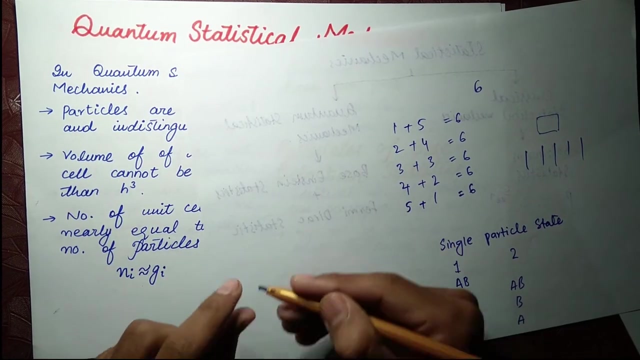 have a more. you can understand a way more better when you understand the fermi direct statistics. but let's have a look. what is this? identical number of particles, for example, we have. let's say here we have identical number of particles, and here the next postulate is any number of. 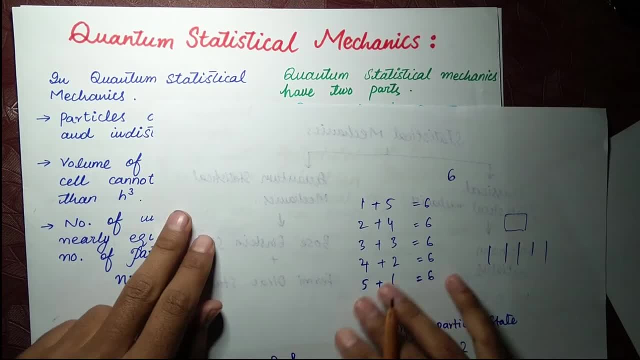 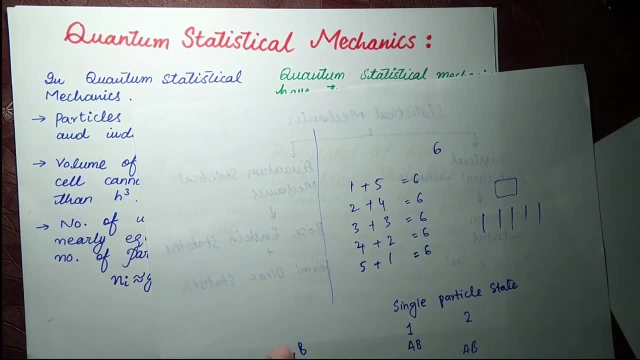 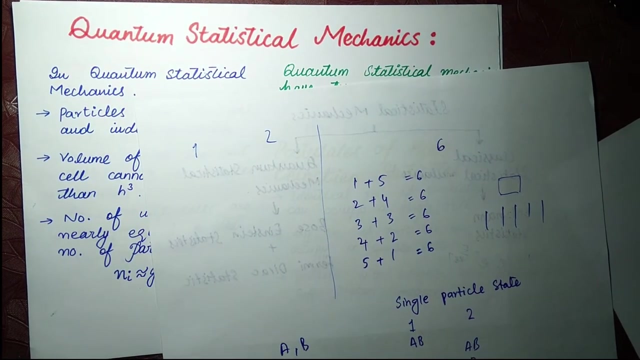 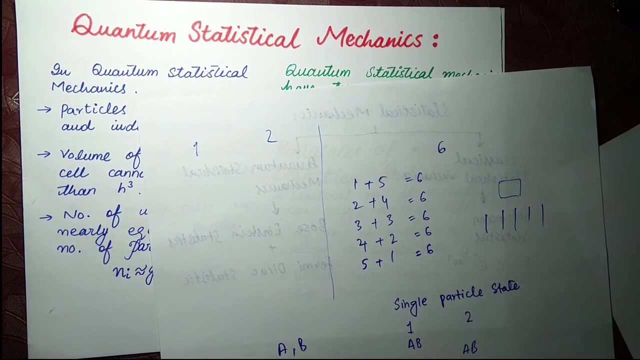 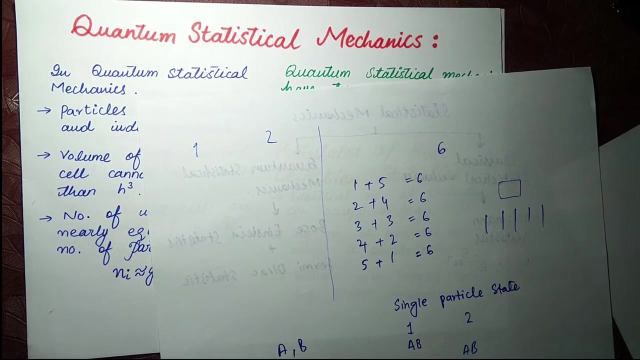 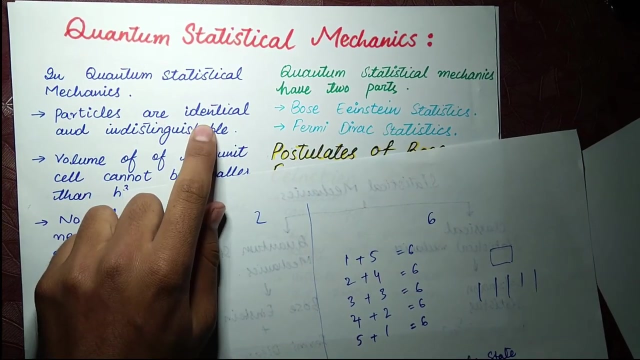 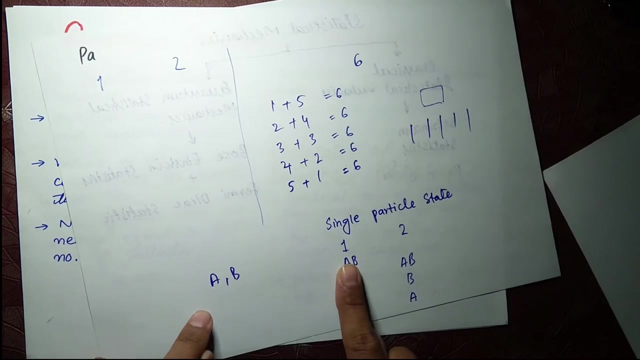 particles can occupy a single cell. so let's say just like this, as we've done before for classical statistics, we do that we have two states, state one and two. we have state one and two, and now this term, this time, our state, our particle are identical but indistinguishable here in the classical. this was, this was the stage i showed you in previous. 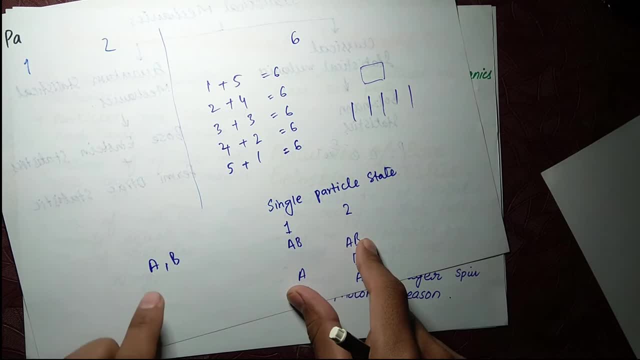 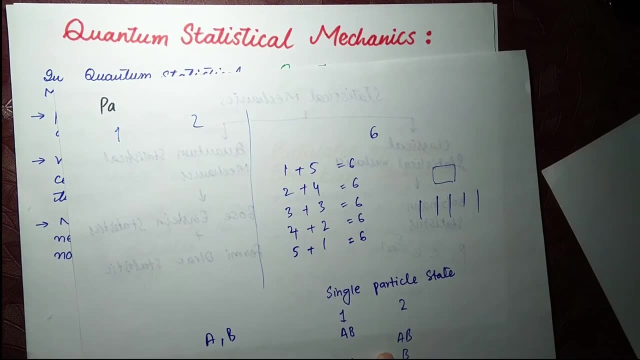 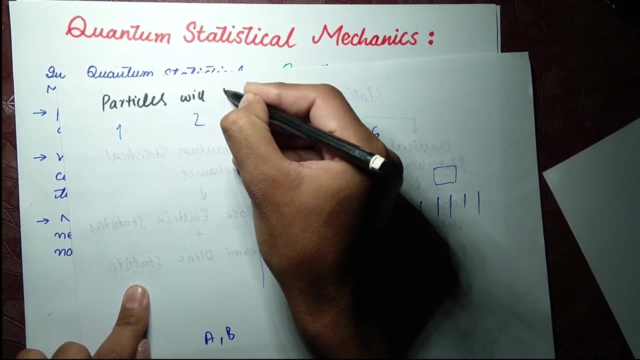 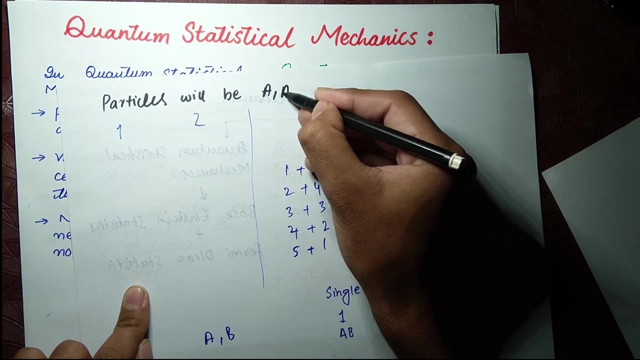 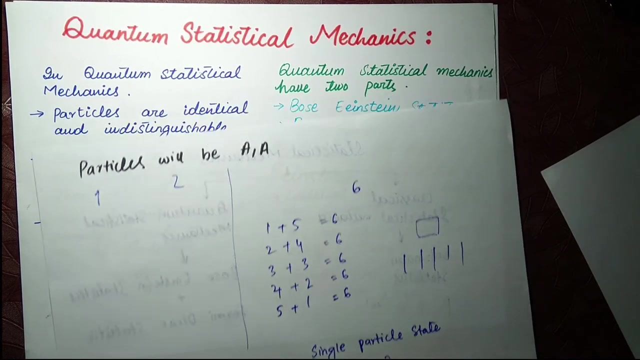 lecture of the classical statistical mechanics, and here it was, particles were a and b, because they were distinguishable. but in this case, now particles are particles will be b, a, and as they are indistinguishable, the other one will also be a. okay, so this time any number of particles can identical number of particles can occupy a single. 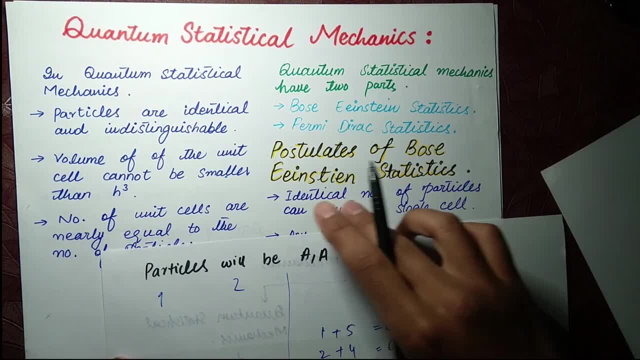 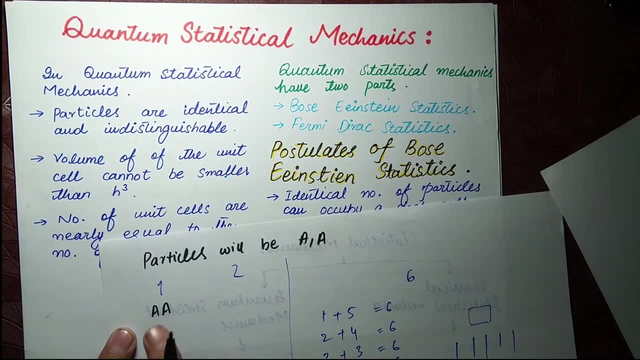 cell. so this, this first, first postulate, says that a and a can be in the same state, and a and a can be in the same state, and a and a and the next can be in the same state here also. okay, and then a could be here and a could. 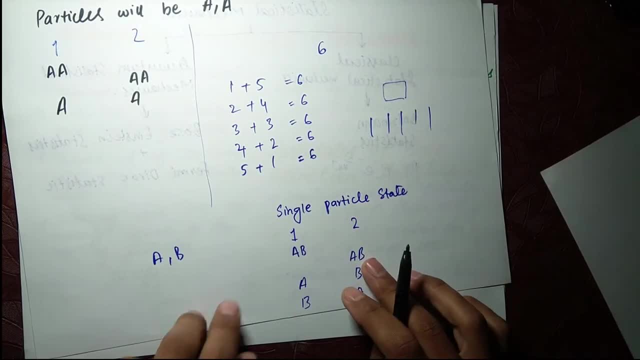 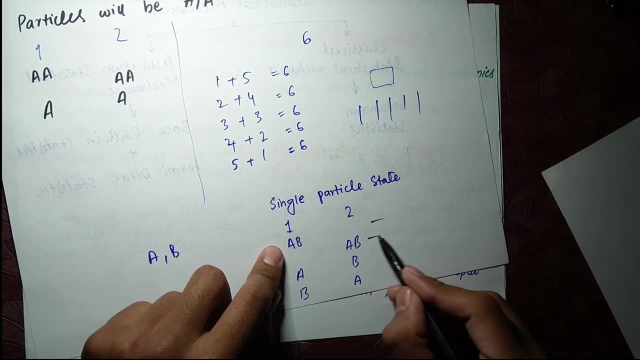 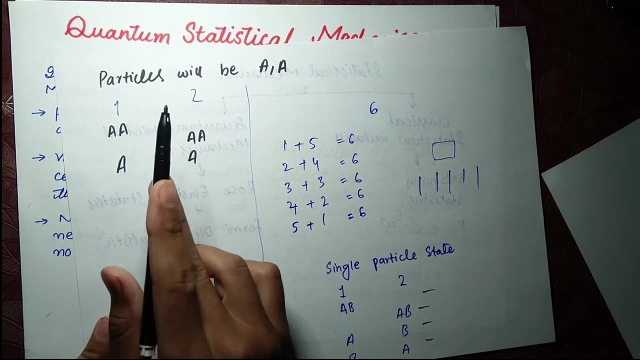 be here. here we have total four states. in the classical statistical mechanics we have total four states: one, two, three and four, this one, this one, this one and this one. but in the case of classical statistical mechanic, in the case of quantum statistical mechanics, we have one, two and 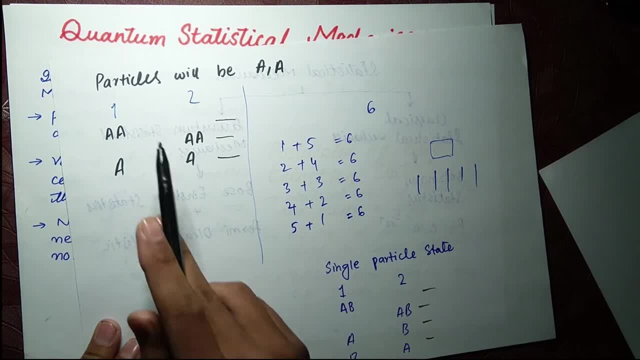 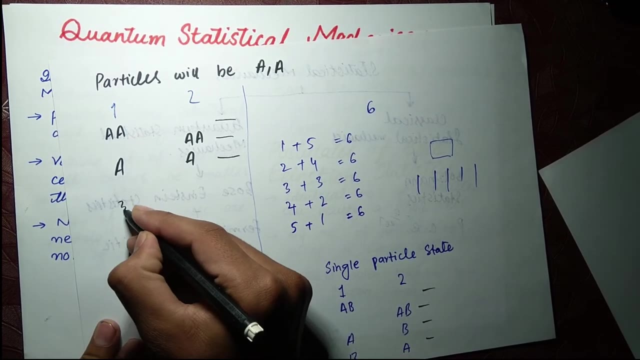 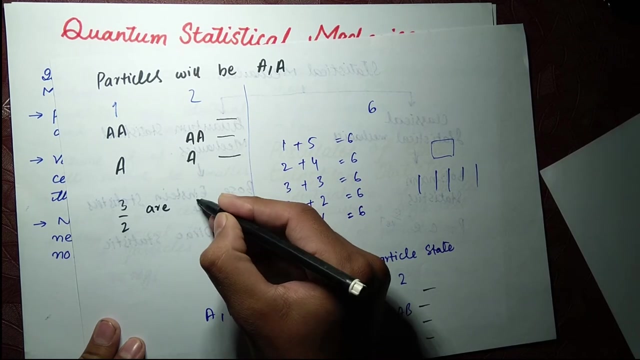 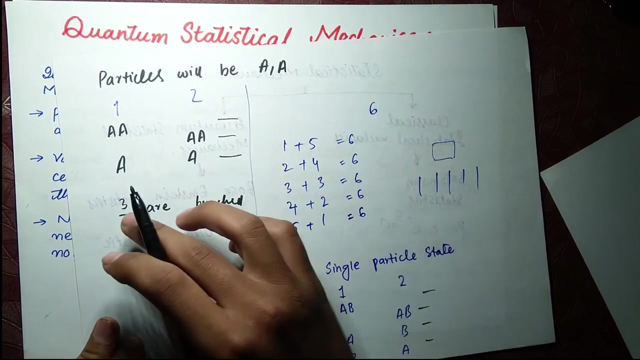 three states. so we can say that in the quantum statistical mechanics, in the boson einstein statistical mechanics, we have total three states for a single particle. we have total three states in which three by two are bunched in the same state. bunched in the same state: a, a and a a, the other two, for out of three. 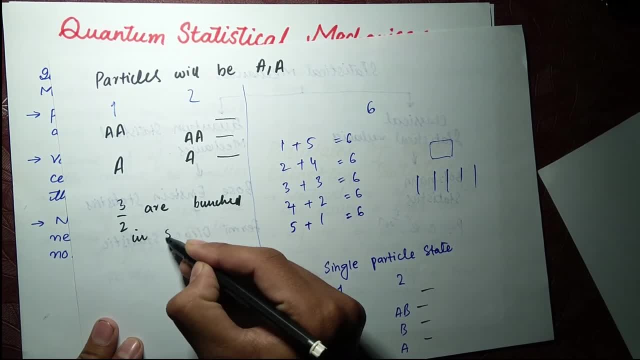 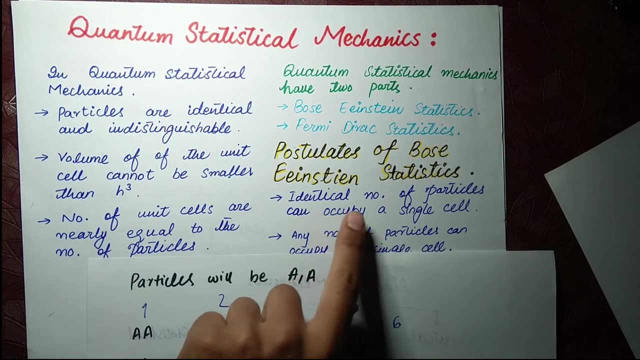 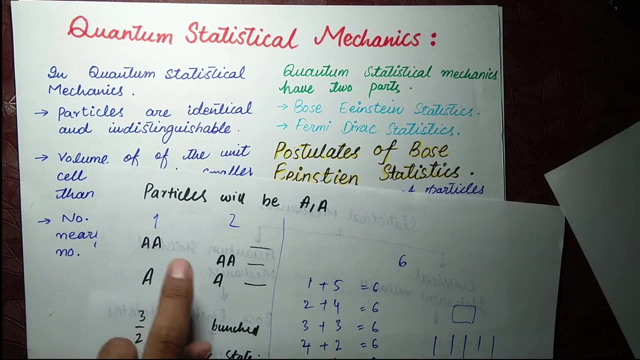 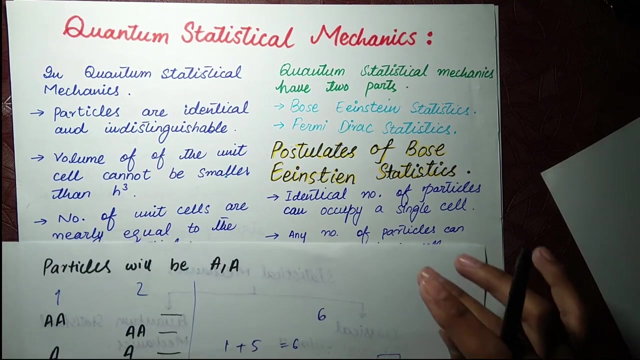 so three by two are bunched in same state. so you understand that identical number of particles that a- a can be together. any number of particles can occupy a single cell. that a- a and a? a could be here. it could be here, it, he could be here. any number of particles can occupy a single cell. when we will discuss the 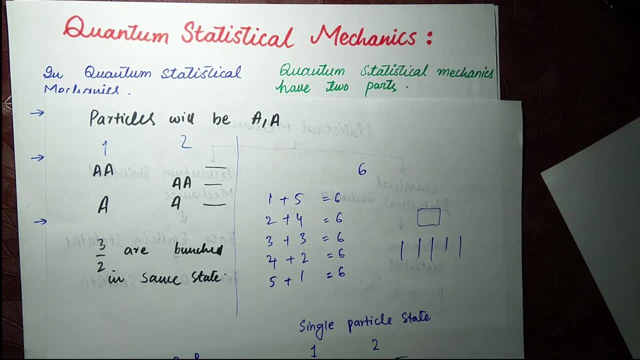 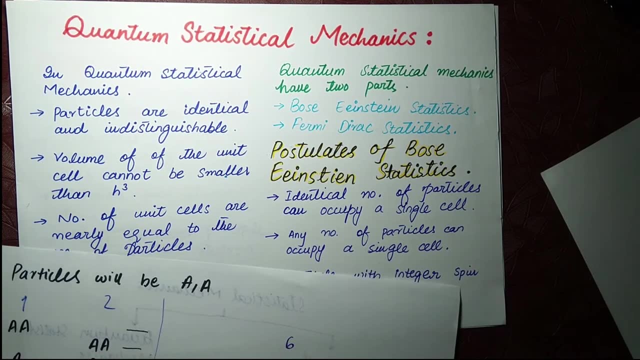 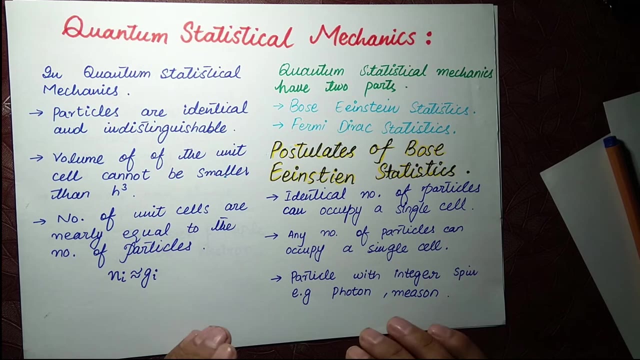 fermi direct. you will understand that. why in the fermi direct these postulates don't apply there, why they don't and when. we will understand that you will get a more clear picture of this. so the particle with the integer spins bosons are have integral spin. why bosons have integral 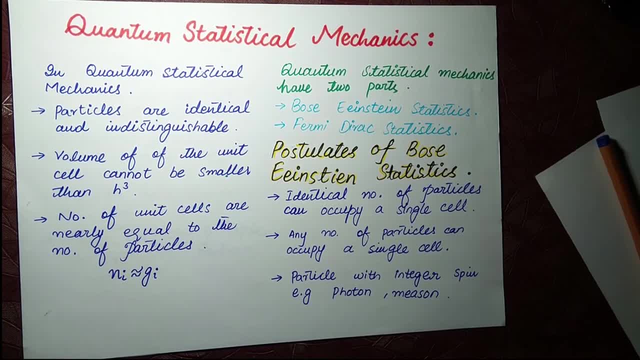 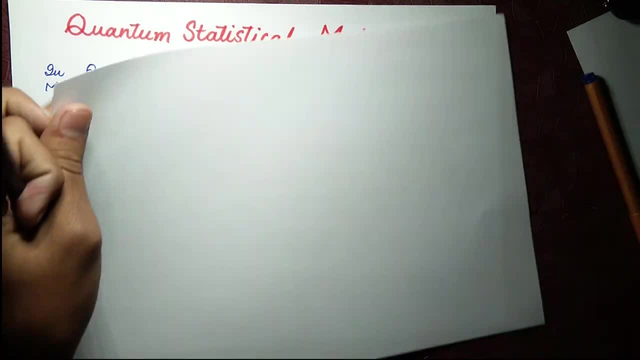 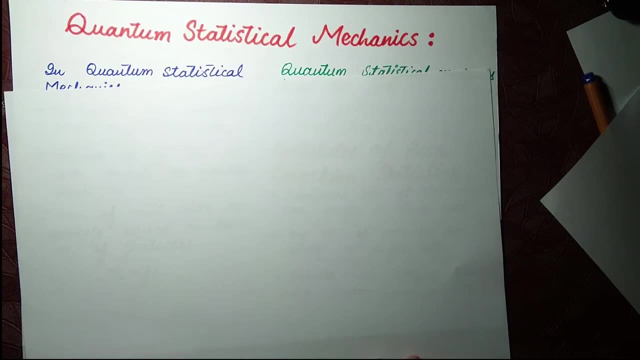 spin because this pin is of positive, negative, one for zero. this pin is positive, negative one, zero, positive, negative, two integers, integers. they have integers so they can fit and they don't have that like in the fermions. and in fermions we have a positive half spin and the 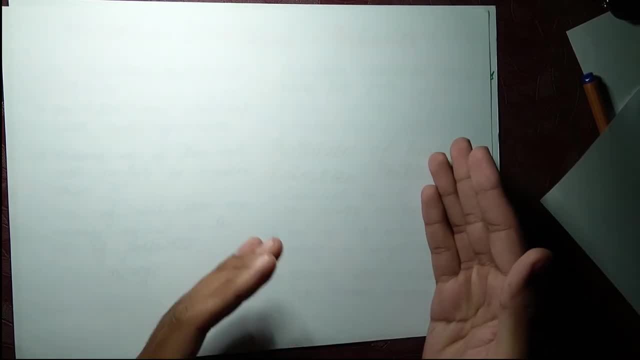 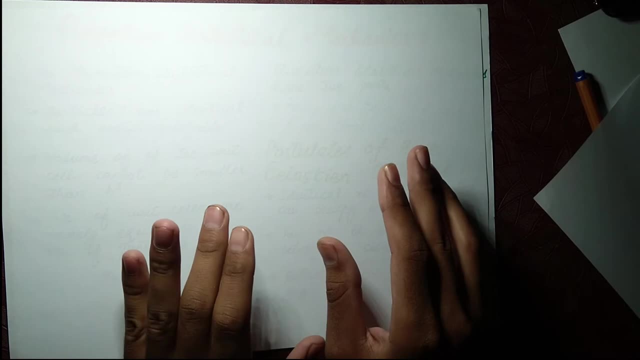 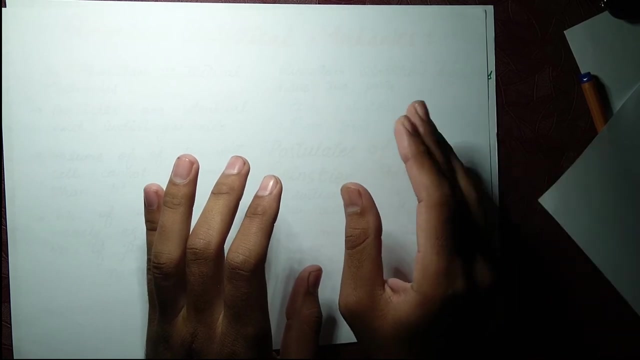 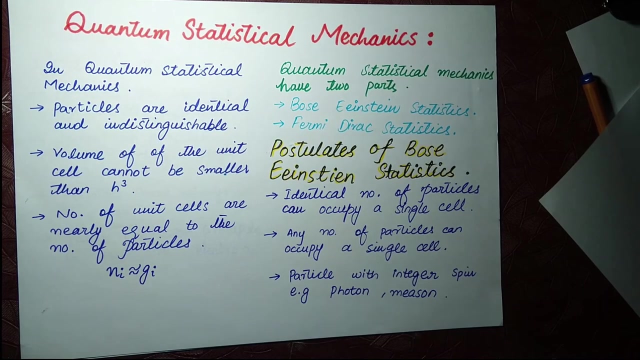 positive, negative, half spin. one is the positive half and the other one is negative half. so they have half integral spin when they have the half integral spin and the poly exclusion principles applies there and we cannot place a positive half with the positive half. but in this case these are the integers, so we can place as much as particles in a, in a single. 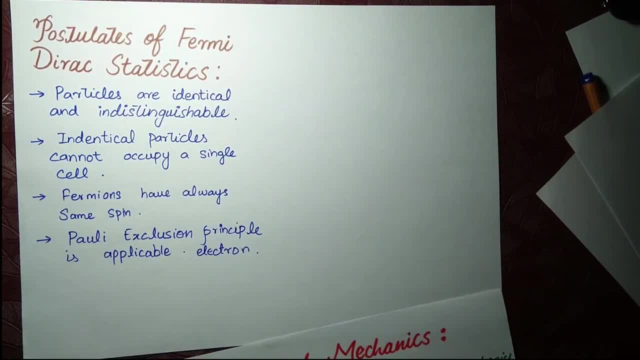 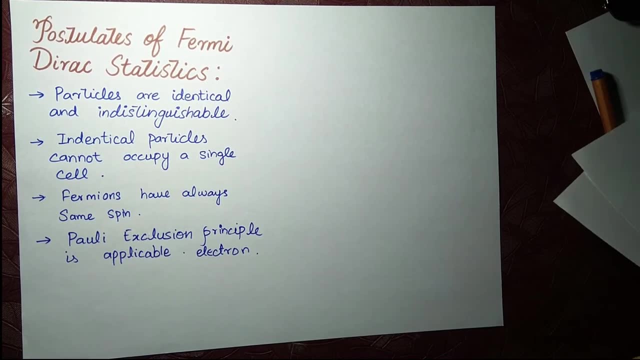 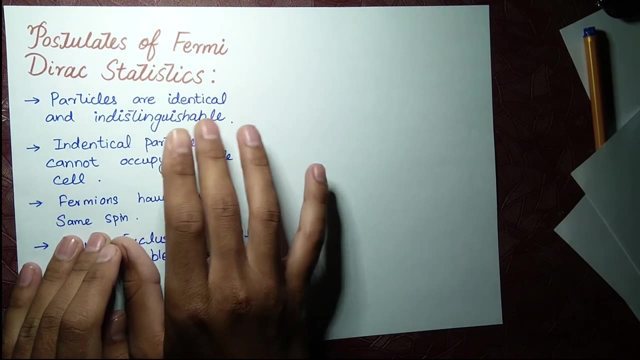 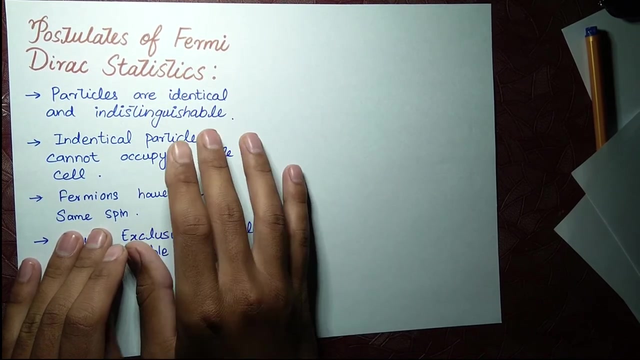 cell. so let's have a look on a fermi direct postulates of the fermi direct statistics. in the fermi direct statistics particles are identical and indistinguishable, just like because this is also a form of quantum statistics. and in the quantum statistic particles are indistinguishable. identical particles cannot occupy a single cell in 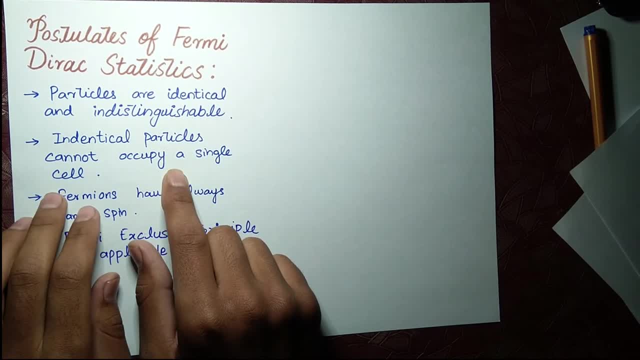 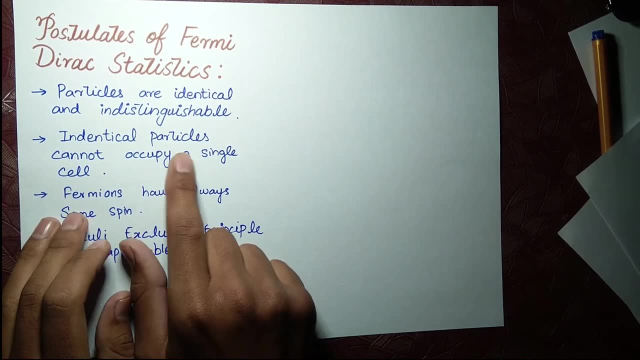 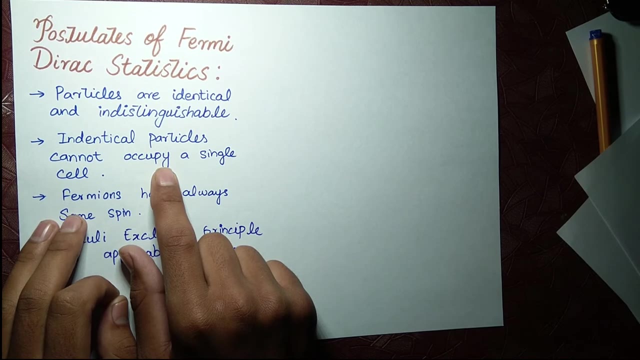 This is the difference between Boson-Einstein statistics and the Fermi-Dirac statistics, that in the Boson any number of particles can occupy a single cell. But in Dirac statistics or the Fermi-Dirac statistics you say identical particles cannot occupy a single cell. 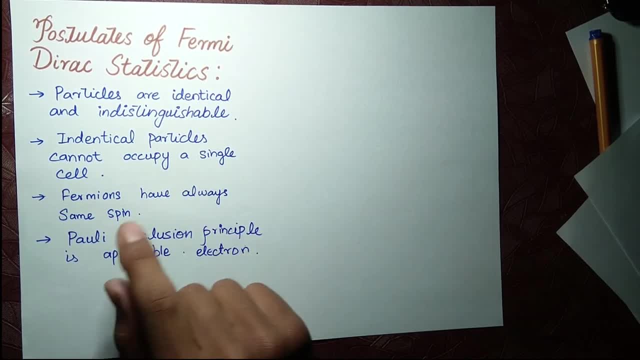 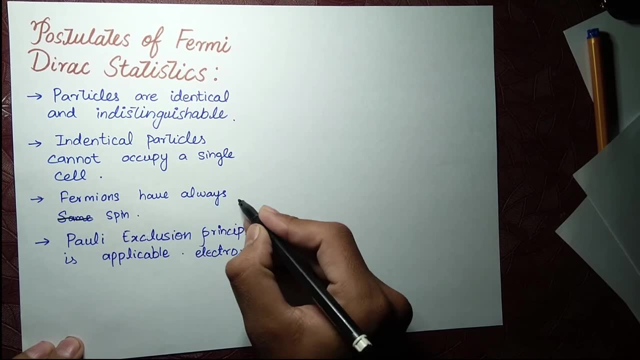 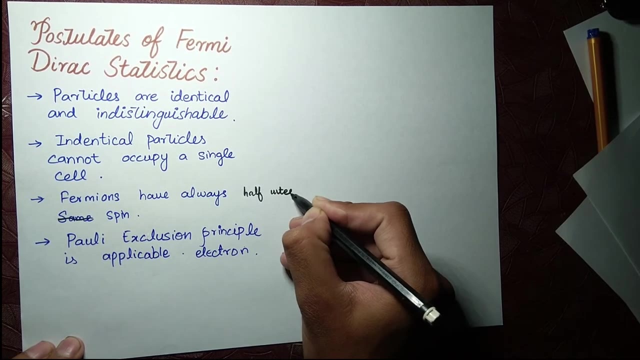 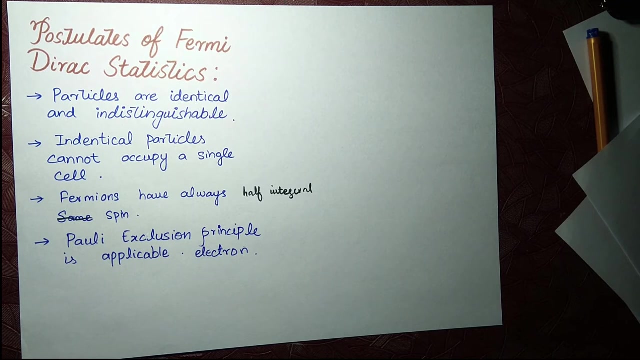 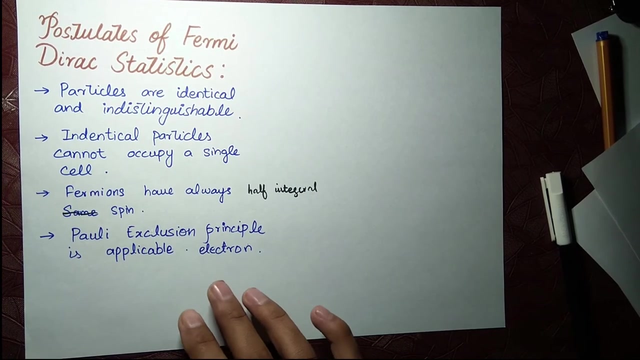 So fermions have always. if here we can say that the fermions have always half integer spin, Half integer spin, Half integral spin, They have half integral spin. So Pauli's exclusion principle is applicable, For example electron. this is the example. 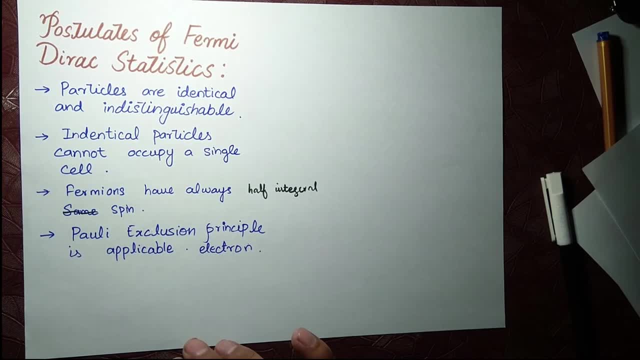 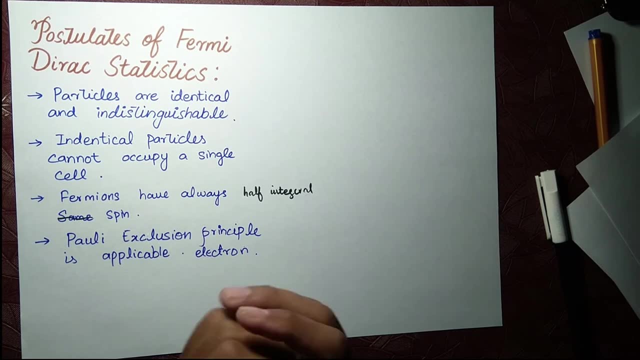 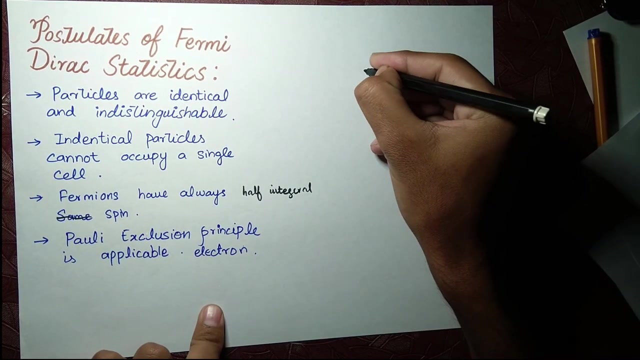 So, as you look in the case of electron Pauli's exclusion principle, when you apply the Pauli's exclusion principle, that you say that the spin quantum number cannot, the atom cannot, have the same spin quantum number in one orbital, For example, that one orbit is having positive. 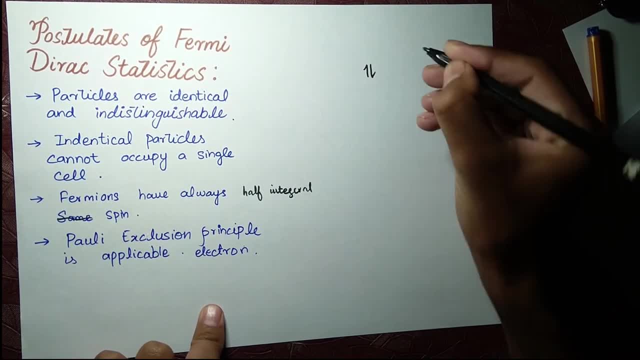 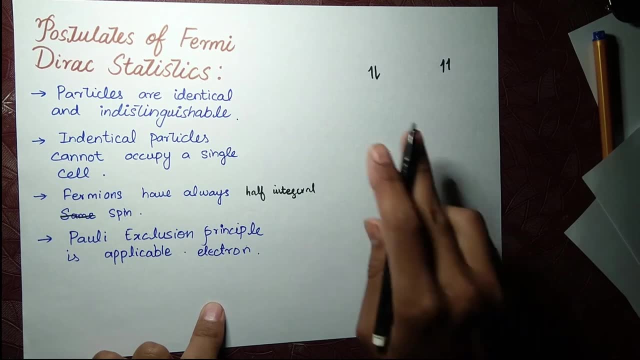 If one orbit is having positive half spin, then the other one will have negative half. You cannot say that this one have positive half and again it will be a positive half. Pauli's exclusion principle says that their spin quantum number should be different. 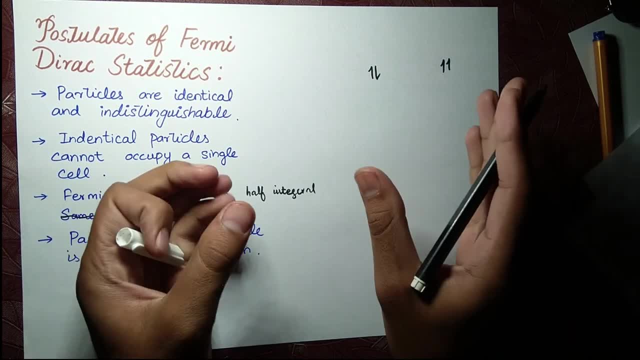 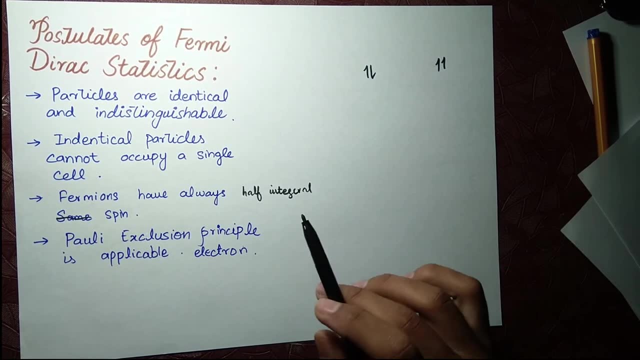 None of the quantum numbers can be same. Two atoms don't have same quantum number. They will differ in their quantum number. So when we talk about the fermions, Protons, electrons, protons and the neutrons are the fermions. 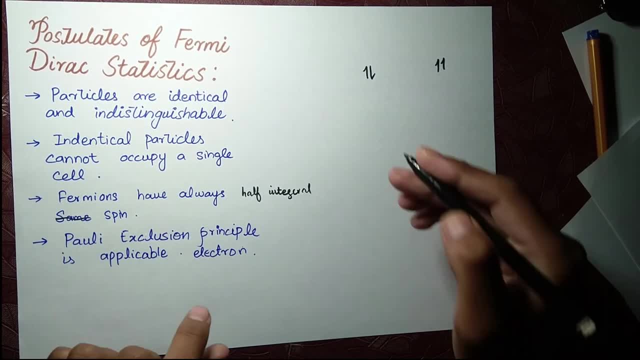 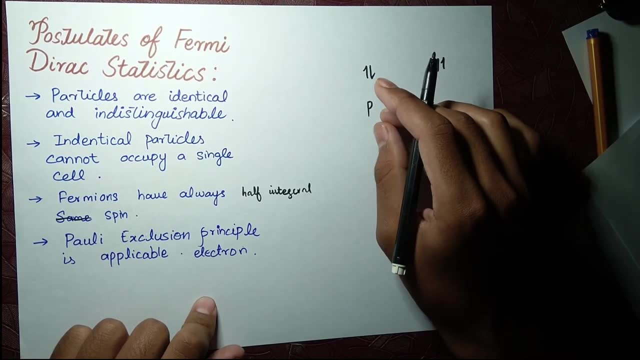 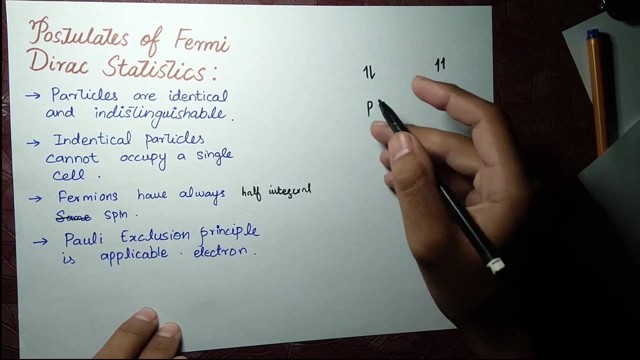 Let's have a look on the fermion that when we talk about a proton. What is a proton? Proton is a nuclear particle. We know that it is present in the nucleus and what it is composed of. So this is the main thing you have to understand: that the proton is made up of quarks. 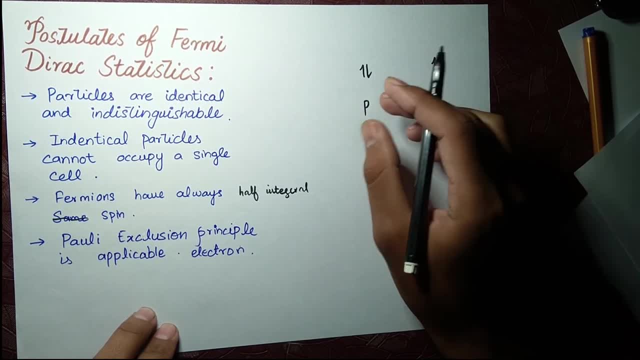 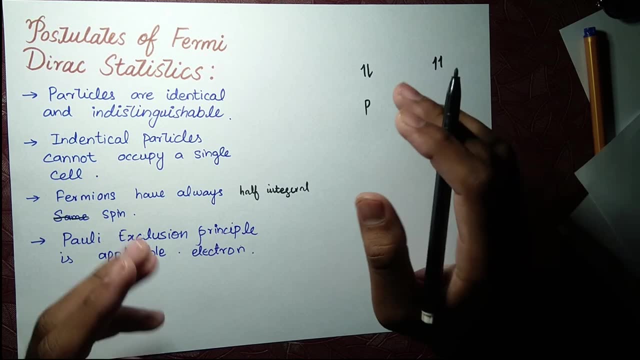 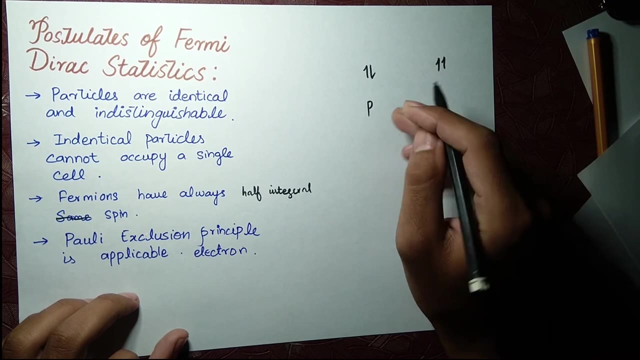 We cannot see quarks individually. We cannot see them individually. We cannot see them individually. They are not independent in nature. They are present in a proton, They are present with a strong binding force and we cannot see them independently. So a quark is of two types. Up quark and down quark. So mainly they are up quark and down quark. In the proton we have two up quarks and one down quark, But in the neutron we have the reverse case of this. We have two down quarks and one up quark. 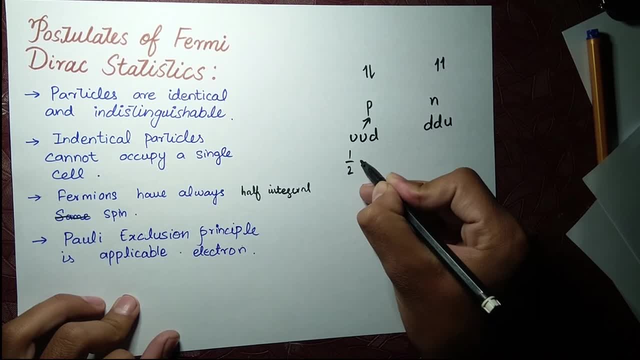 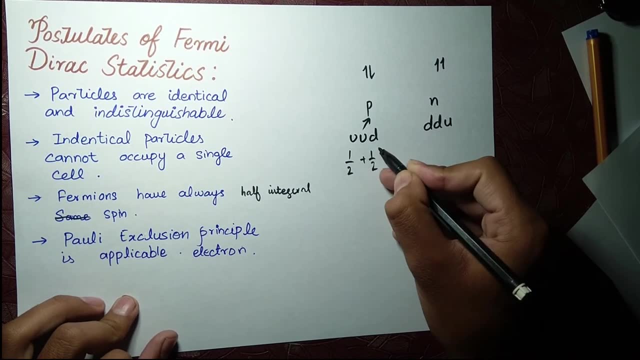 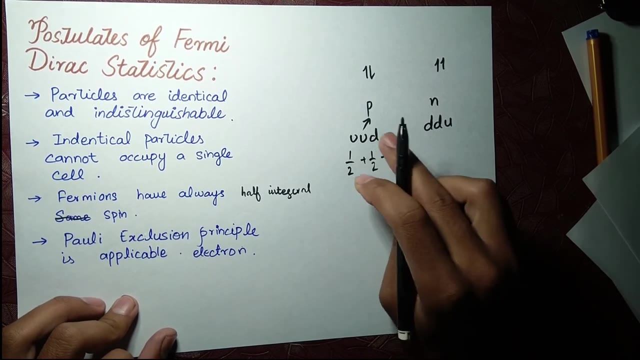 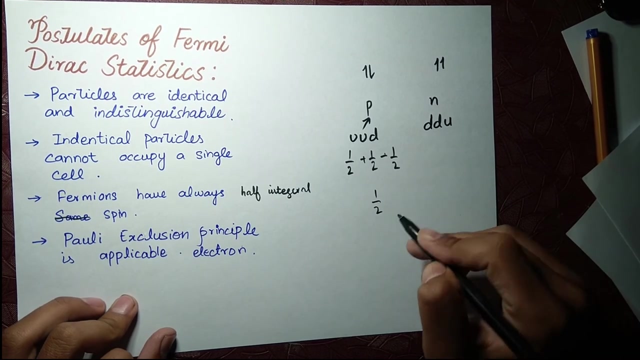 This one is equal to plus half plus half. Up quarks means they have the positive half and half spins And the down quark means they have the negative half spin. So because of this positive half, You can see that overall spin of this will be the positive half. 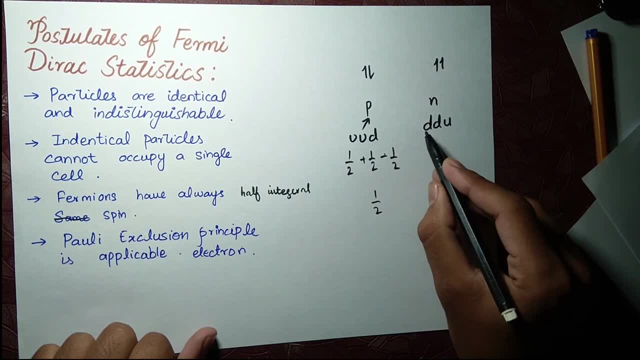 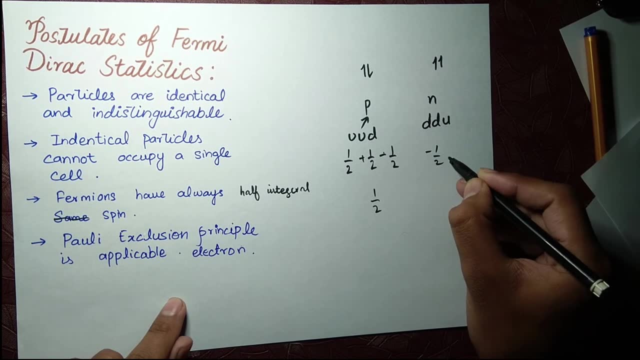 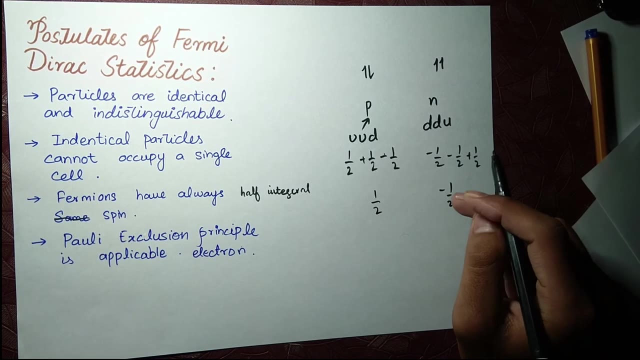 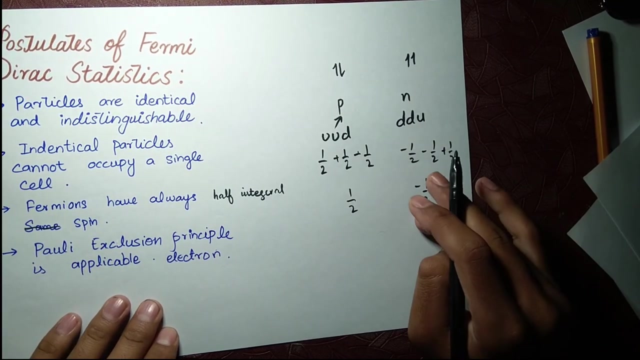 Then the neutron here have down, down and down. This will be have negative half, negative half plus positive half And the overall charge will be the negative Overall charge. I am saying Overall spin will be the half negative half. So you can see here that this is positive half. 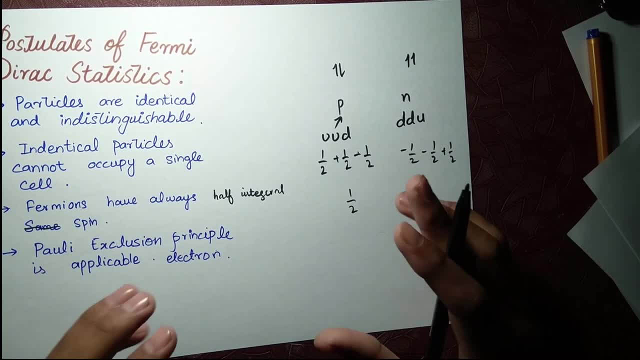 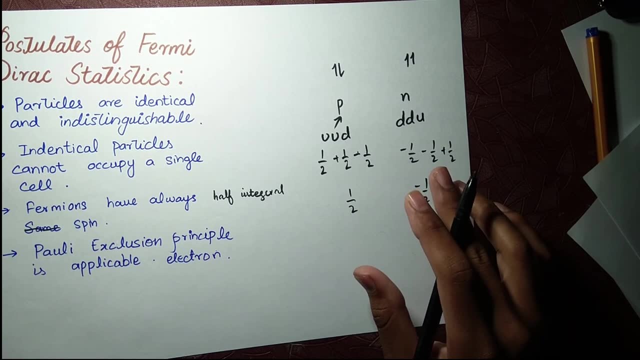 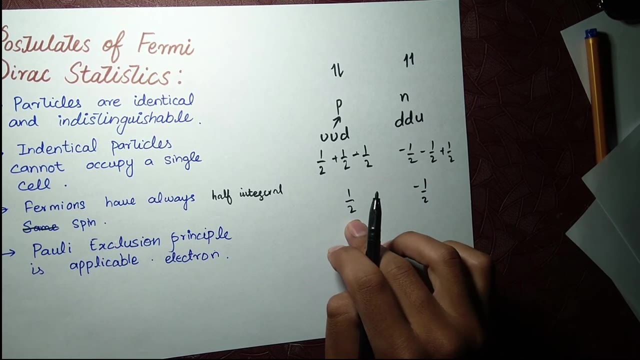 This is negative half Proton and the neutron. overall their spin will be conserved. So I think you understand what a fermion is. Just like electron, Electron have a positive half spin also and the negative half spin, But in the proton we have a positive half spin. 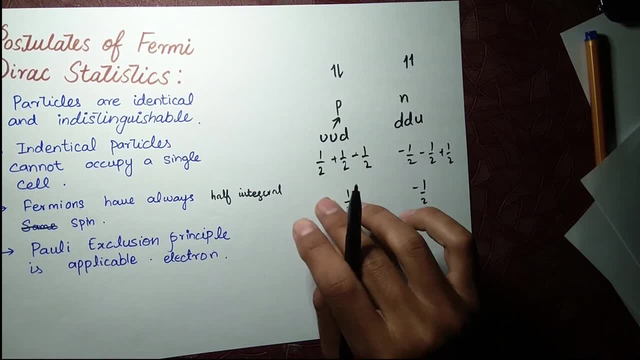 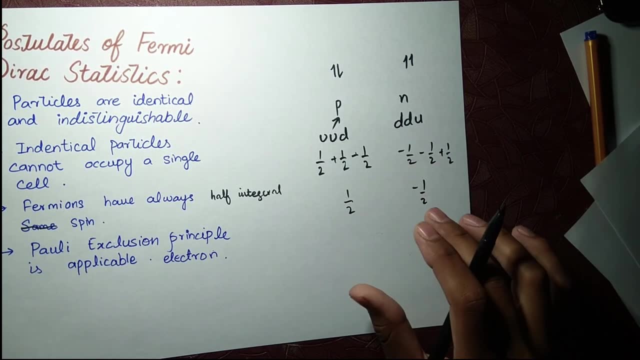 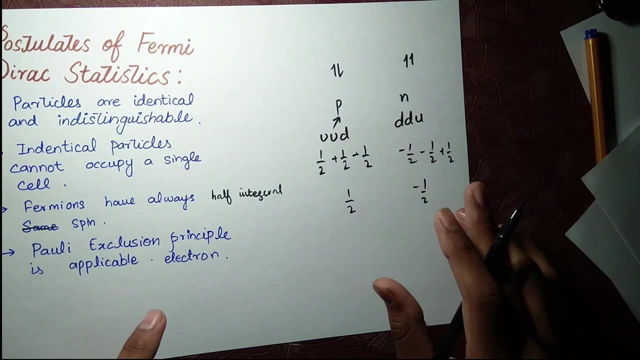 And in the neutron we have a negative half spin Because they are composing of quarks, And two up quarks here and two down quarks here And overall spin. you can see, you can understand what fermion is. Now you can understand, you have a picture in your mind about fermions.